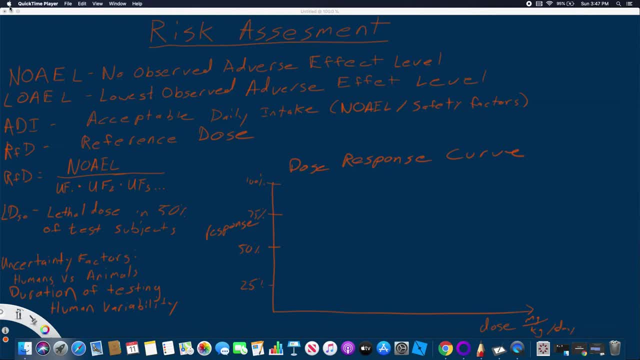 we usually use some terminology based on the number of responses per population of test subjects, And so just kind of jumping right into the terminology, here we have our NOEL and sometimes we use some terminology based on the number of responses per test subjects. So what this means is: 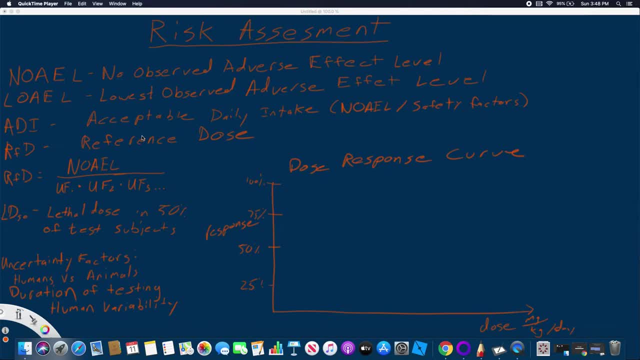 this is a concentration. this is the highest concentration where there was no adverse effect in the test population. So if you're testing mice, they didn't get cancer, they didn't have cancer. sometimes you have low L, which is lowest observed adverse effect level, and this basically. 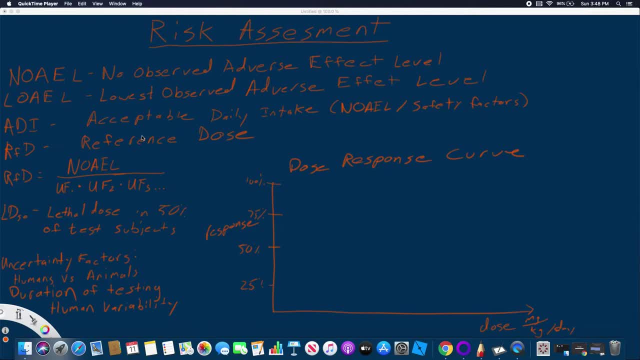 means. whatever your data are, this is the lowest level that showed um some kind of adverse effect, cancer damage, whatever reproductive harm. Normally you don't want to use low L, That's you basically only use that if you don't have a no L. Obviously you want to use the LE If you would. keep using it as the main factor in your selection, but a cyber threat. so if you don't have this username, pull a feels. well, now it's pretty. permission that, but you need to go with Which lead to the BONUS: K ra rophBl SyrianL que no BarryWhat does the binoculars lead toый? We don't have to. you know who it is, but primary. 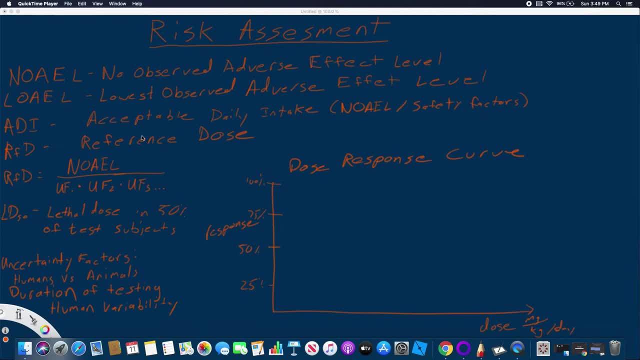 will collect them afterwards to know which in which um at reste can actually use your name if something that comes to like you, And so, anyway, What I'm not going to go over are some of this you want to use. no L, whatever would be. give you some confidence that you're not going to. 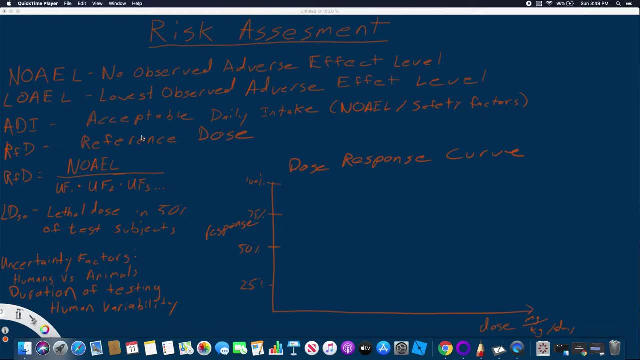 harm the population, right, But sometimes that's not available. And then what used to be used in risk assessment was the ADI, or Receptible Daily Intake, And this would be the no L, if available, or low L, if it's not divided by a safety factor. Well, we've modified how we 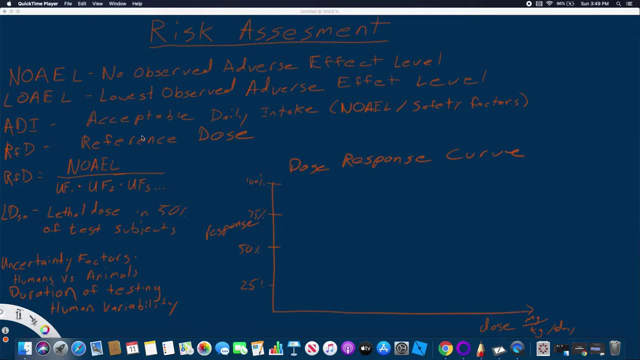 look at safety factors. We've kind of gotten more specific in terms of safety factors, So what you're probably going to see nowadays is the reference dose, the RFD, And so the reference dose is your no L or low L divided by your uncertainty factor, And you can have a lot. 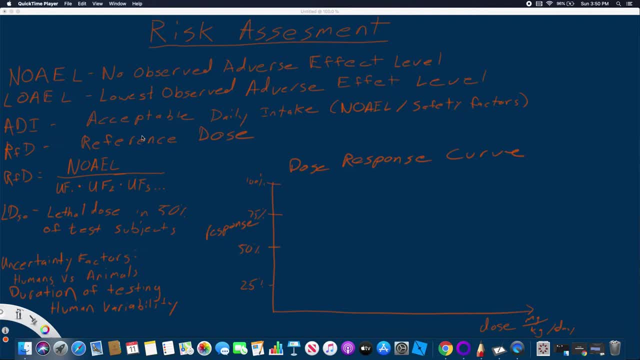 of different uncertainty factors based on whether you know. you're probably going to have a factor of 10 right off the bat, just because humans tend to be very different. right, And we do a lot of these studies with the idea of an adult human in mind. But what? 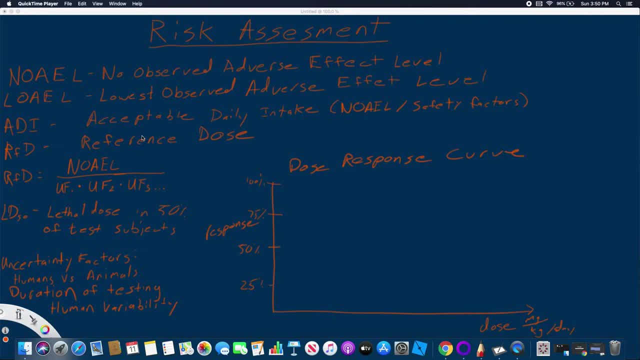 about children right, They have a very low body weight. They also have developing organs which are much, much, much more susceptible to damage while they're developing. So there's a lot of variability there that if you want to try to protect people, you need to add in a safety. 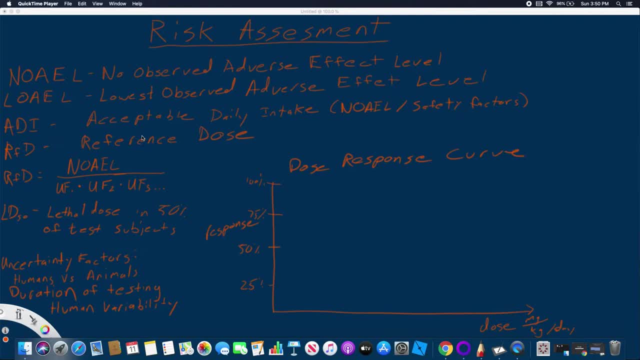 factor. based on that alone, There could also be uncertainty, because most of the time we're extrapolating data from animal studies. We can't test humans. I mean, that's you know. obviously that's not ethical. So we tend to do studies on animals and we try to say: 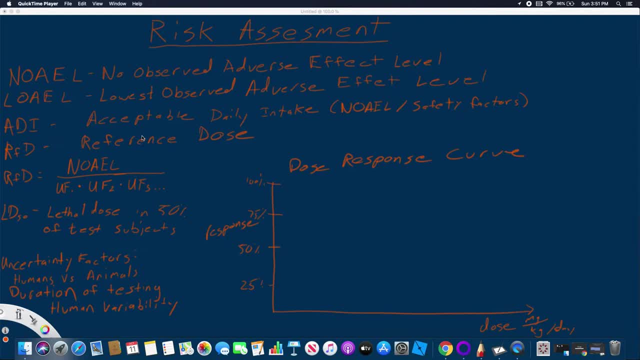 like: well, it harmed an animal, so it's probably going to harm a human too. But we don't know how those exactly translate right. So we need to be you know. if we wanted to protect people as best as we're able, we need to be you know, include that uncertainty into our factors when we're. 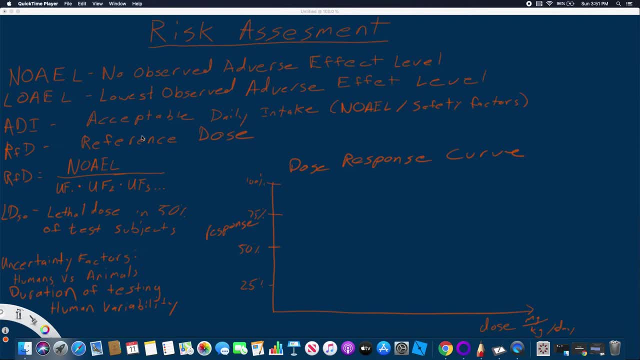 talking about translating animal studies to humans. Also, duration of testing tends to be an issue when we talk about studying animals. A lot of these times, the animals don't have the same lifespan that humans do, Or we don't, you know, if we're. 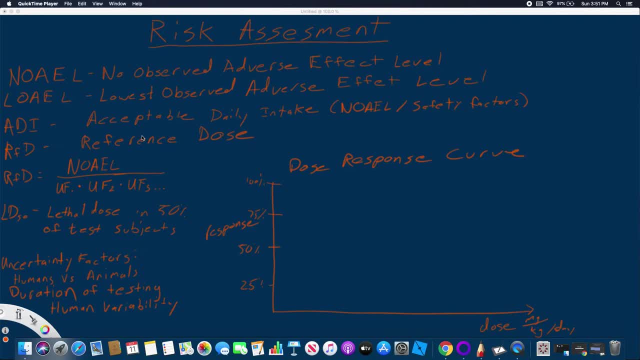 talking about a carcinogen over a person's lifetime of 70 years roughly, then we can't wait 70 years to get the results right. We need these quicker so we can make decisions now. We need to accelerate these studies and extrapolate them out over a longer period of time And 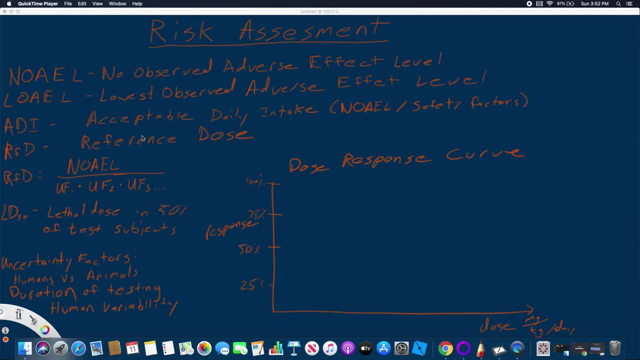 obviously that's going to cause more uncertainty. So there's a lot of uncertainty factors here And we account for that by basically applying factors of 10, usually of uncertainty- to lower what we would consider an acceptable daily intake basically. So that's basically. 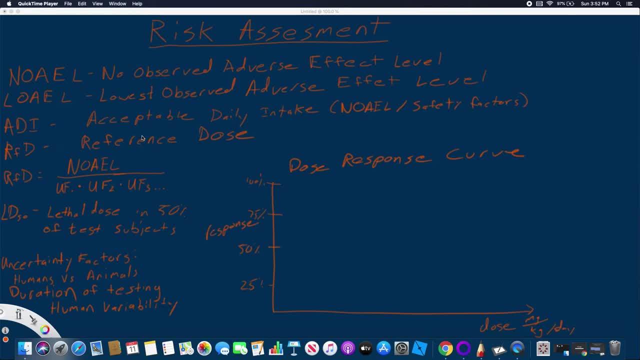 how risk assessment works In terms of the FE exam. you know any of these topics could come up. they could be oh, and also the lethal dose. So this is kind of comes back to variability, something you might get asked about: lethal dose. So lethal dose is, or LD50 is, what is the lethal dose? in 50% of test subjects. So you know, obviously, even with my own tests, I'm going to be able to do that. So you know, obviously, even with my own tests, I'm going to be able to do that. So let's. 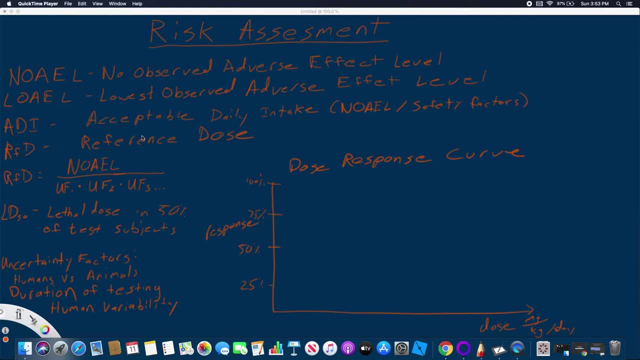 do that. So let's do that. So let's do that. Okay, so, let's do that. Okay, so, let's do that. So let's do that. If you have 100 mice, you're going to have variability. If you have 100 mice, you expose. 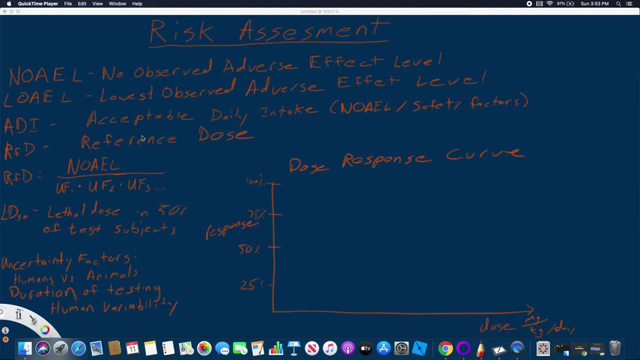 them to some concentration. you know what would cause death in 50% of the test subjects. That's kind of how lethality of a contaminant is determined. you know basically on what causes death in 50% of test subjects. 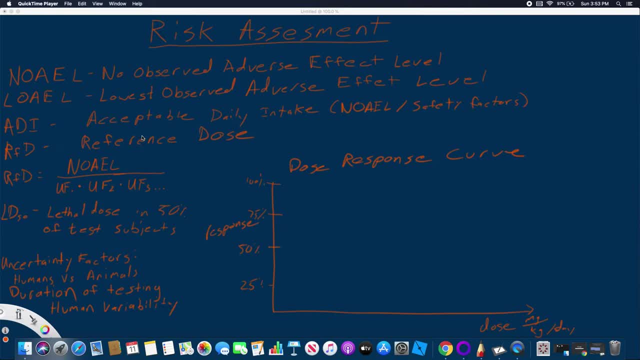 Okay so. So another thing you're probably going to see on your FE exam- or I'd be surprised if you didn't- is going to be the dose response curve, And so what this is is you have increasing dose on the. 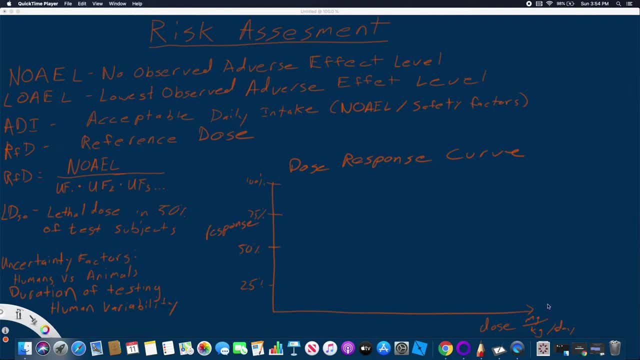 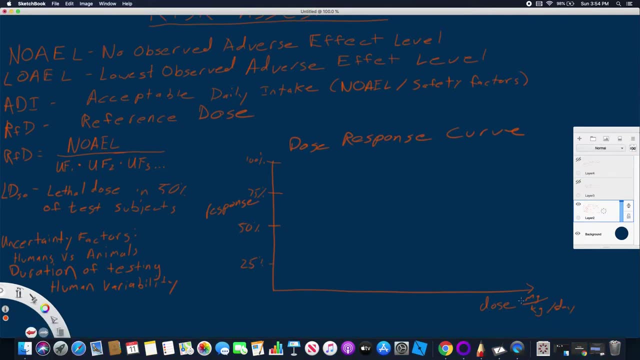 x-axis, right. So here here you have increasing dose and increasing dose on the x-axis. So milligrams per kilogram of body weight per day is your exposure And then response. Response is basically the percentage of test subjects that had a adverse effect. 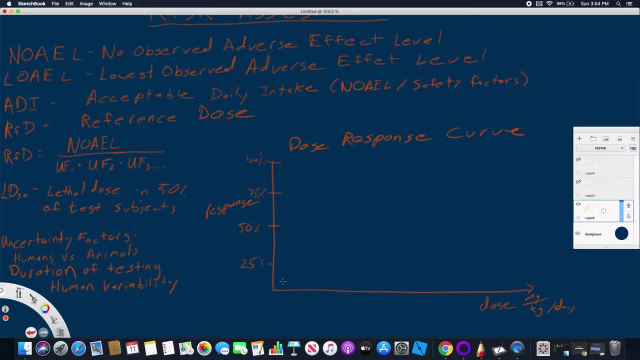 And so what you're probably going to see, and what you would want to see if you were conducting these experiments, is something like: okay, we've got nothing, We've got nothing, We've got something, We've got something. yeah, we've got something. So, basically, here is your slope, but this would be your no L, This is your no observed adverse effect level. right. 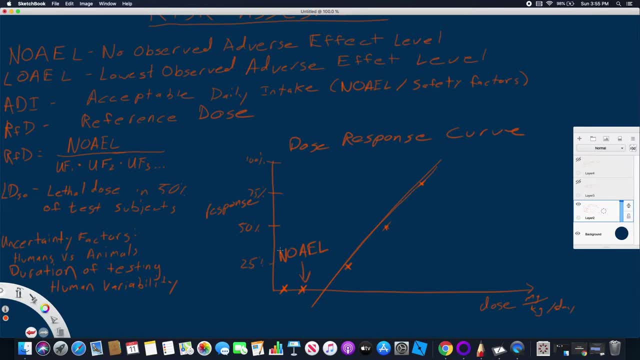 Because if you were using whatever this dose is, there was no observed effect. right, There was nothing. nothing happened, Nothing that you could observe actually happened Now over here. this would be your lowest observed adverse effect level, So hopefully you would have. 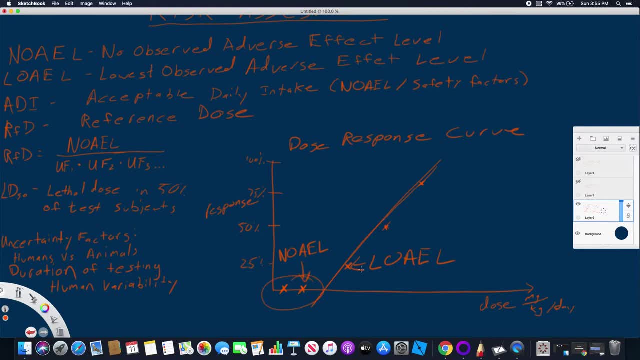 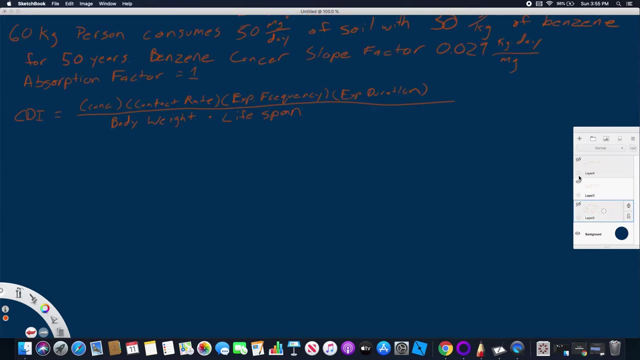 You would have these data, but if you didn't, then you would use your low L And yeah, I mean basically that's all there is to it really. So we'll move forward, Okay. so a couple of examples. 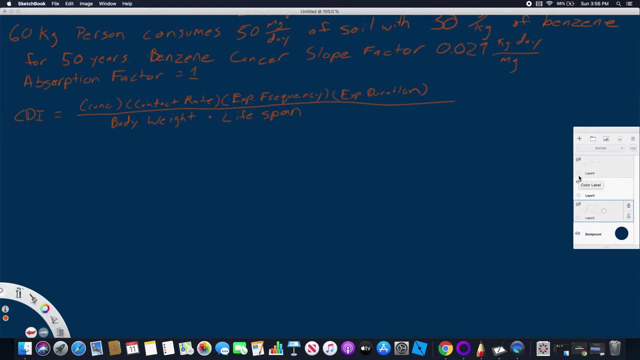 If we have. So probably you're going to see some kind of You know cock Calculation for what is like cancer risk or what is the CDI or something, some kind of calculation for risk assessment, And it's probably going to be something along these lines here. 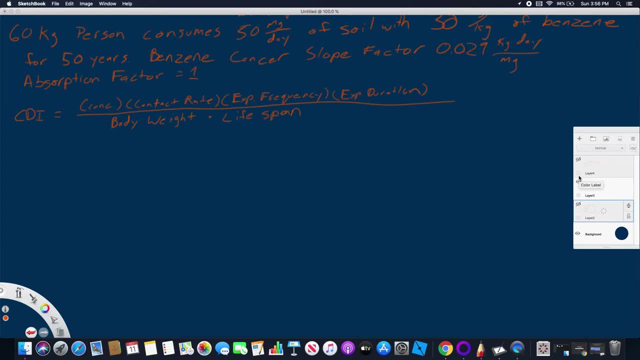 Now remember there's a difference between cancer risk and non-cancer risk, basically non-carcinogens- because with cancer risk it's always, always, always, always averaged over a lifetime, Where with a non-cancer risk it's just based on exposure duration. 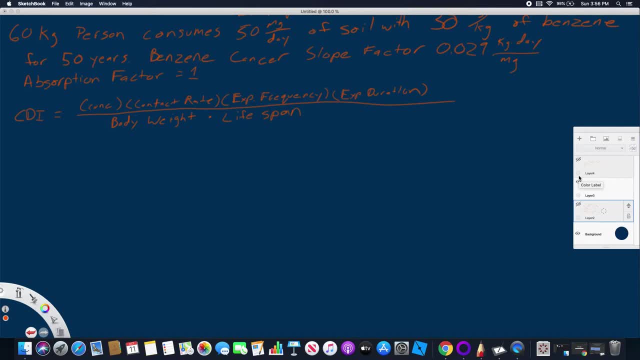 So that's one thing to keep in mind. So in this case we're talking about a cancer risk. So we have a 60-kilogram person. They are consuming 50 milligrams per day of soil. I know that sounds disgusting, but basically you do breathe soil every day. 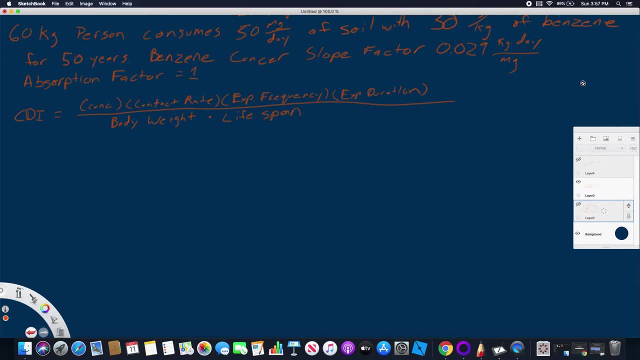 It just It's part of life. And Can I get this to stop being weird? I don't know. So, 30 milligrams per kilogram of benzene for 50 years- Okay, so what we're probably talking about here is a worker who worked well, in this case, every day for 50 years. 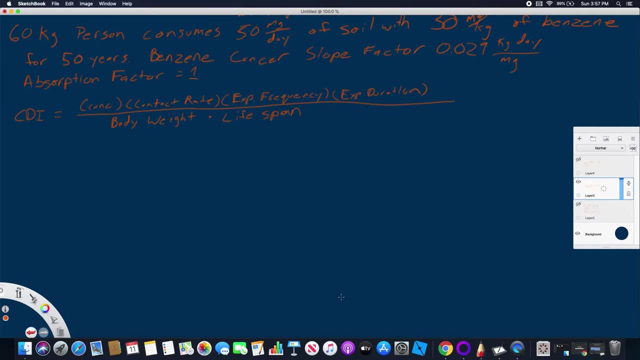 And they were breathing in soil that was contaminated with benzene. The benzene cancer slope factor is 0.029.. And it's kind of inverted from consumption, So it's kilograms days per milligram And with an absorption factor of 1.. 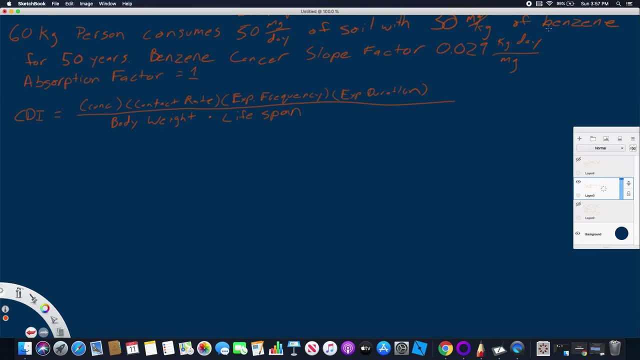 So in this case it means that all exposure was absorbed. Basically, we're not going to limit it based on some kind of- like you know- exhalation that wasn't absorbed, or whatever. It's fully absorbed. Okay, so we have a CDI. 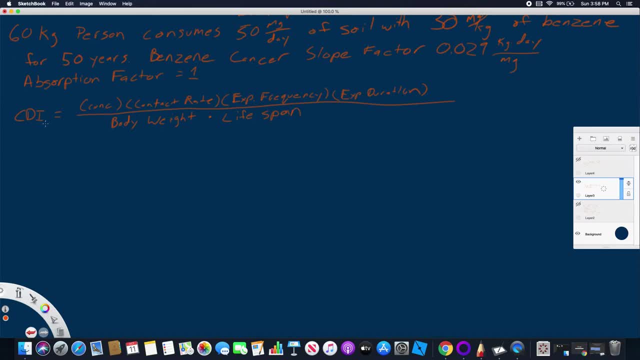 This is your chronic daily intake And this is equal to your concentration. In this case, 50 mil- Yeah, 50 milligrams per day, sorry Times. your contact rate, which is 30 milligrams per kilogram. So we have the exposure of soil. 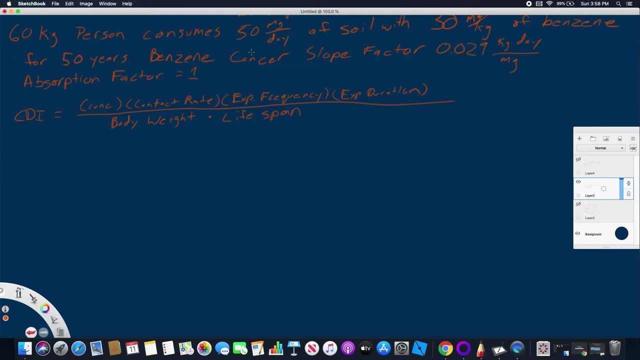 Times, the actual benzene in the soil. Your exposure frequency, which in this case, because we didn't specify it, we're going to assume this is every day. It's seven days a week. This could be different if it's like a worker. 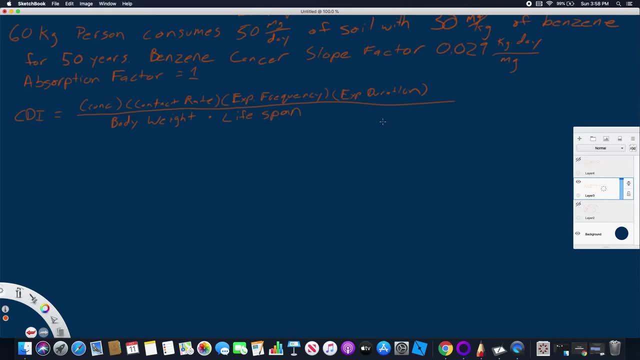 It might say five days, you know, per week, So you'd have to basically five-sevenths of a year. Or it could be something like: Often municipalities use risk assessment for handling toxic waste sites by ironically building recreational facilities like a soccer field, right? 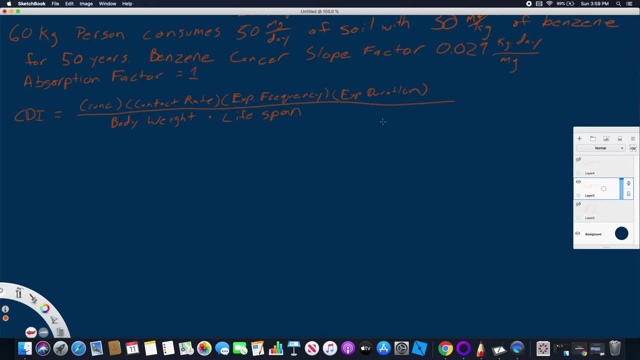 And, if you think about it, how often do you play soccer? Maybe twice a week, right, For a couple hours. So your exposure frequency is really going to be quite low And from that your CDI is going to be very low, right. 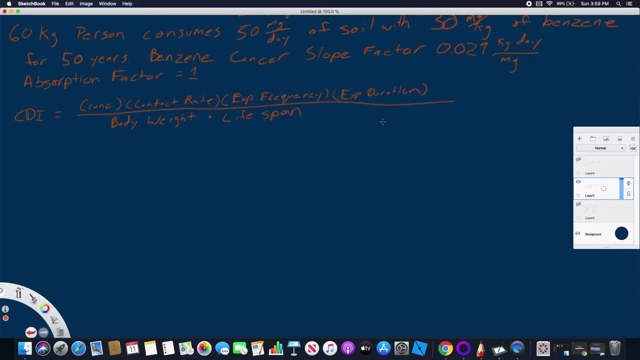 So, So, that actually is a strategy often used to deal with toxic sites: Basically make them into soccer fields. So okay, So, blah, blah, blah. Exposure duration is going to be, obviously. how long were you exposed? 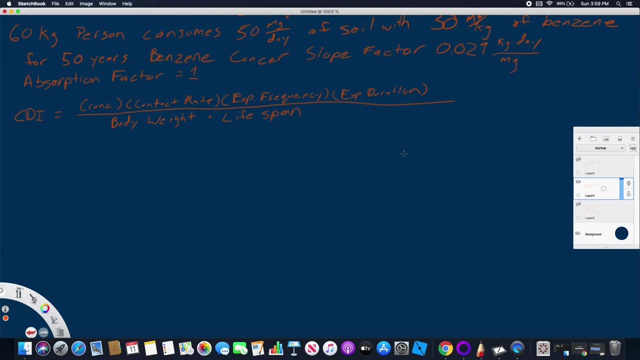 In this case 50 years. So you think about, like how long were you working? And then you're going to average that out based on a person's body weight, And so usually we'll use an average. 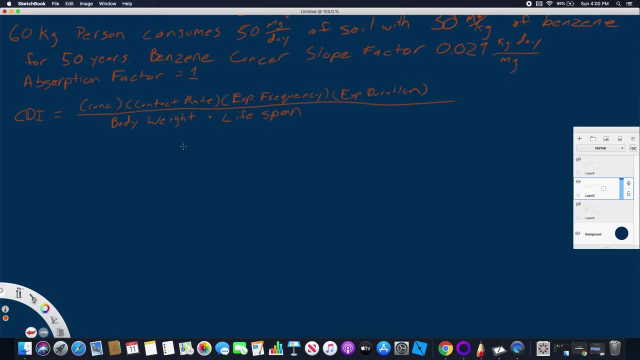 Male adult body weight of like 70 kilograms. It might give you some different value, but you know, whatever, If it doesn't give you something, then it's probably going to be 70. And then lifespan, which again is an average value. 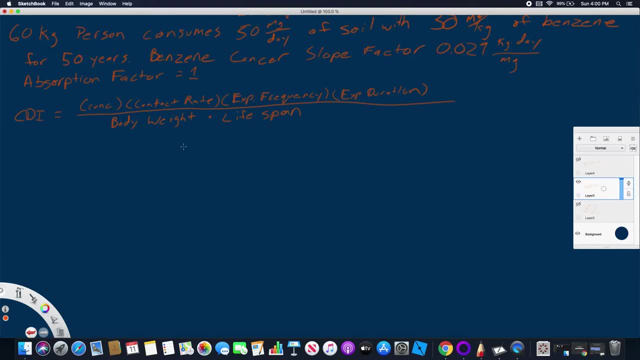 Typically it's 70 years, 365 days per year. So if we Just checking my time, Wow, Okay, 15 minutes already. So if we look at this, we're going to have 50 milligrams per day of exposure. 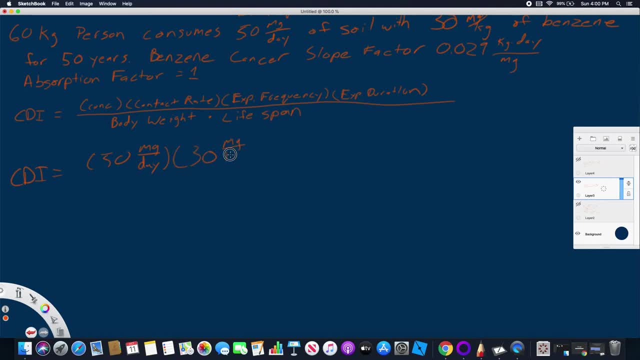 We have 30 milligrams per kilogram of contamination in the soil. We want to convert this from kilograms to milligrams for our body weight. We have 365 days per year of exposure And then we have 50 years of like how long the person worked or whatever. 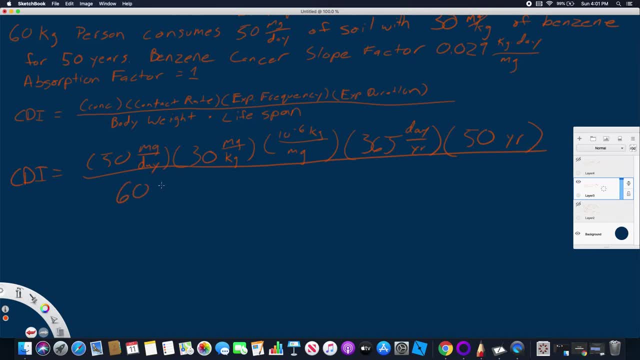 All right. So then, since we said, in this case, for some reason, we're talking about a 60-kilogram person, that's our body weight, So we have a 70-year lifespan And 365 days per year that they're alive, I would hope. 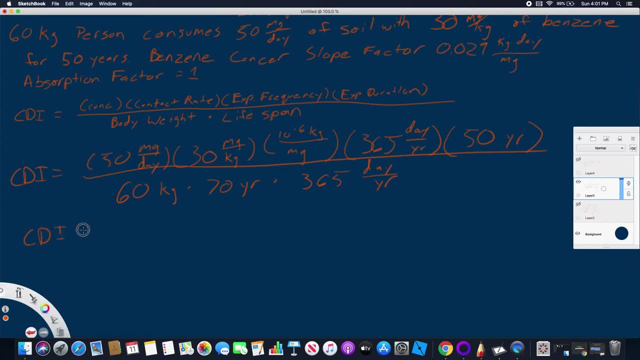 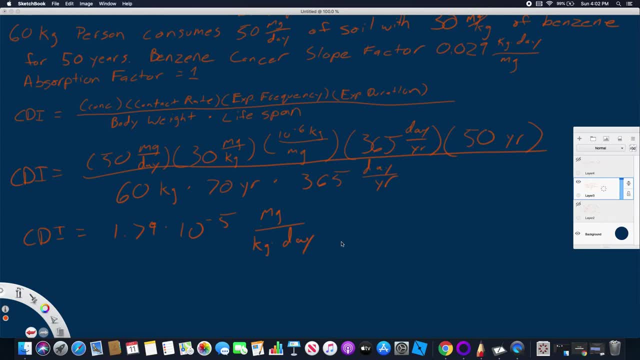 Ooh Ooh, Ooh Ooh. Okay, So that's the chronic daily intake. This is basically the average amount of contamination in a person's body, averaged by their body weight over their lifetime and exposure, because that's you know how you deal with cancer. 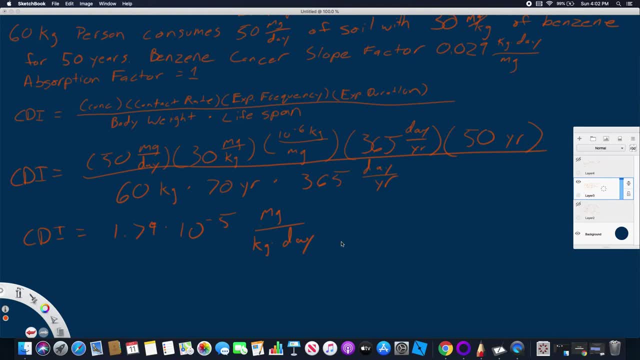 It's not. There's no safe exposure for cancer, right Right. So any amount of exposure is going to affect your average exposure per lifetime. It's kind of a Maybe a little bit confusing, but basically any exposure is going to affect your cancer. 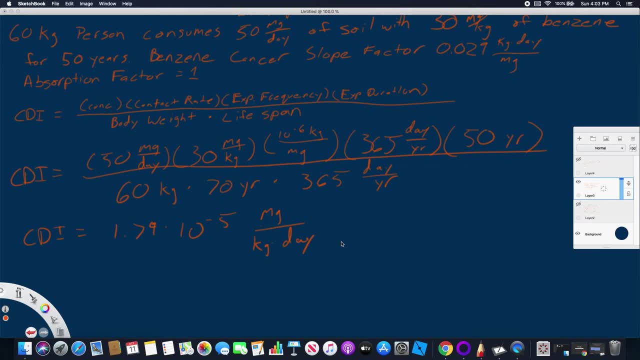 risk over your life, unlike non-cancer, which, basically, if you don't damage your cancer, if you don't damage your organs, you're probably fine. So okay, Your risk is going to be equal to your CDI times your slope factor. 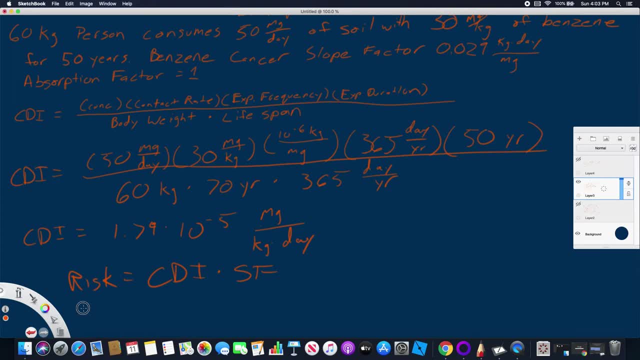 Now we haven't talked about, We haven't actually used that yet, but risk. your actual risk here, or calculated risk, is going to be 1.79 times your slope factor. Okay, So that's going to be 1.79 times your slope factor. 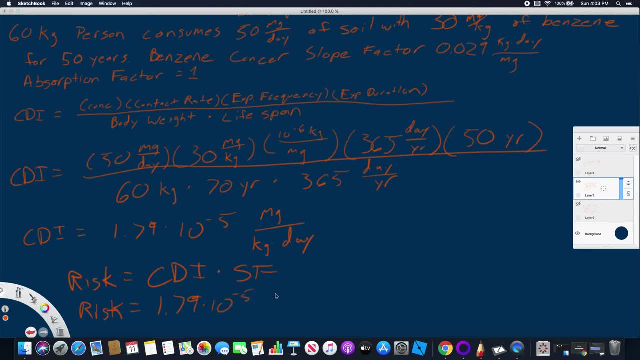 Okay, So that's going to be 1.79 times your slope factor. Okay, So that's going to be 1.79 times the negative fifth milligrams per kilogram day times our slope factor, which is 0.029 kilogram days per milligram, which in this case is 5.18 times. 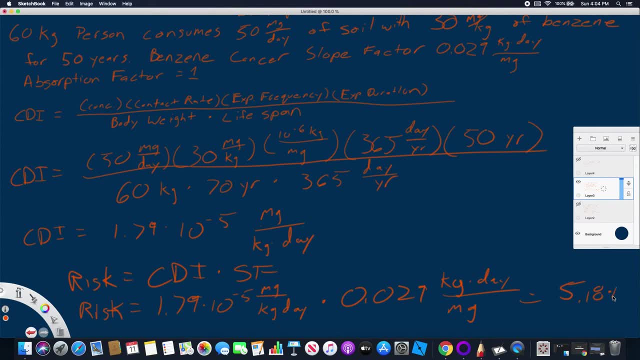 your slope factor times 10 to the negative 7 and this would be considered an acceptable risk. so that's actually something else that might come up in the exam is what is acceptable risk, and acceptable risk is usually one per one million or one additional cancer occurrences. 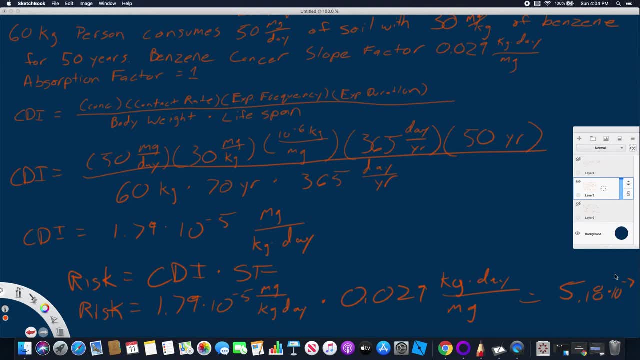 per million exposures. so if you have a city that has a million people and you have something in the water supply that may cause cancer, if it only causes cancer in one person over a lifetime, that would be considered acceptable. that's basically generally, at least in the US. how? 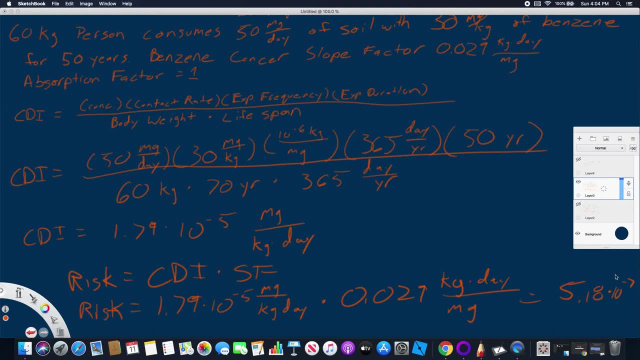 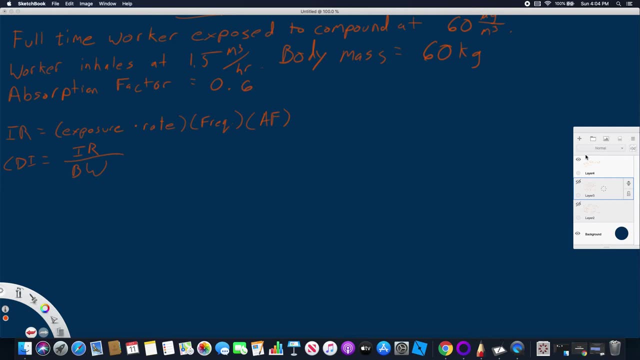 cancer risk is sort of evaluated okay. so one more example here: if we have a full-time worker exposed to a compound at 60 milligrams per cubic meter of work space and the worker inhales at a rate of 1.5 cubic meters per hour, which is 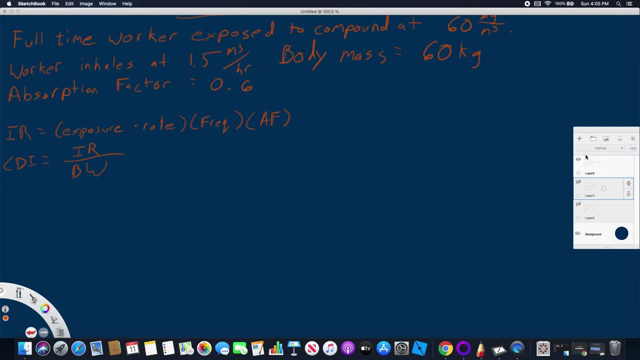 somewhat, maybe a little bit- elevated, but maybe if you think about a worker that's maybe doing some kind of physical contact with a person that might cause a load or a háMă cuánt Women worked inches off by 2st at 375 pounds per hour. extra, wennes корабIGRAMs added up to 30 grams per qualcúber per hour, which is somewhat, maybe a little bit elevated, but maybe if you think about a worker that's maybe doing some kind of physical contact with a person that's simply fast moving and getting those Bronco doctors볤ºdolfish is unique as well. 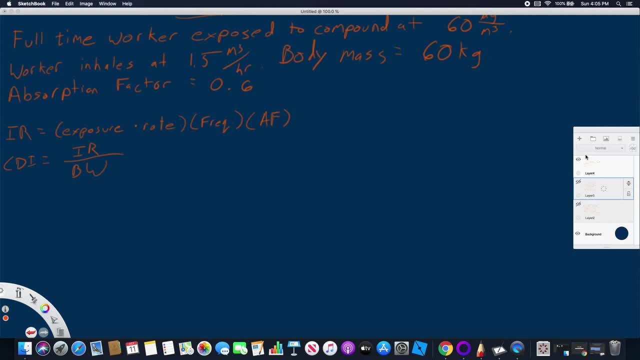 work they might be breathing quicker. so a more active worker might breathe at 1.5 cubic meters per hour with a body mass, again, of 60 kilograms and in this case an absorption factor of only 0.6, so they're only absorbing 60% of the 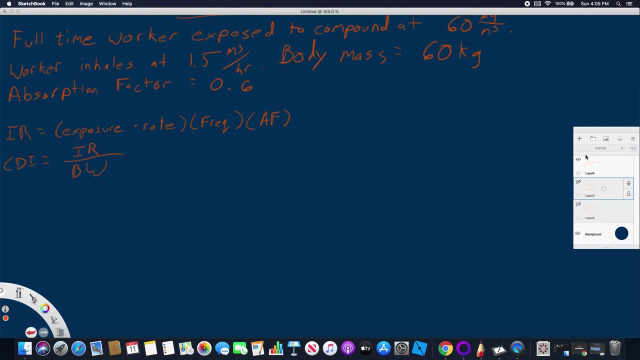 concentration into their body. so in this case, we want to take a look at the intake rate, which is going to be the exposure, which is the 60 of this. I'm sorry if it's actually micrograms. can't quite see what that is, but that's. 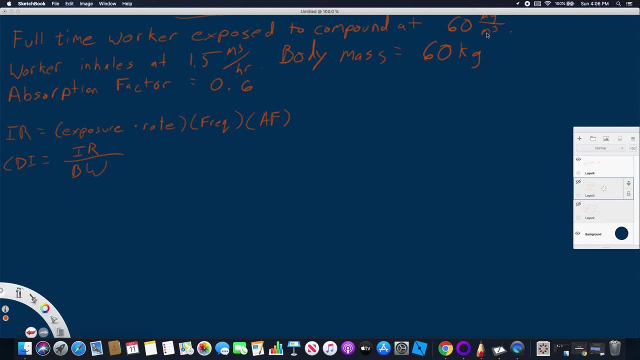 actually micrograms per cubic meter, for this example times the rate of exposure, which is 60% of the body mass. so in this case, we want to take a look at the, which in this case, is going to be 1.5 cubic meters per hour times the. 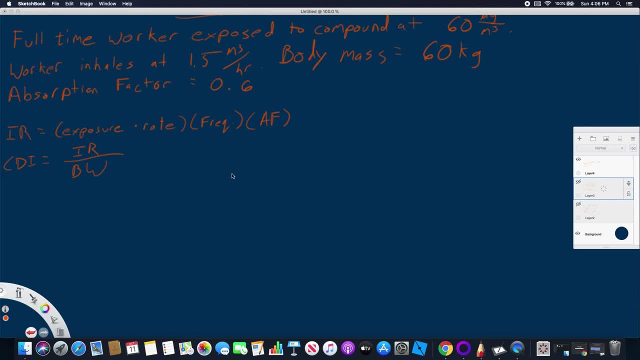 frequency, which, in this case, we're talking about a worker. so we're going to assume that this is going to be a 40 hour work week and that that's going to translate to eight hours per day. all right, and then we're going to have an. 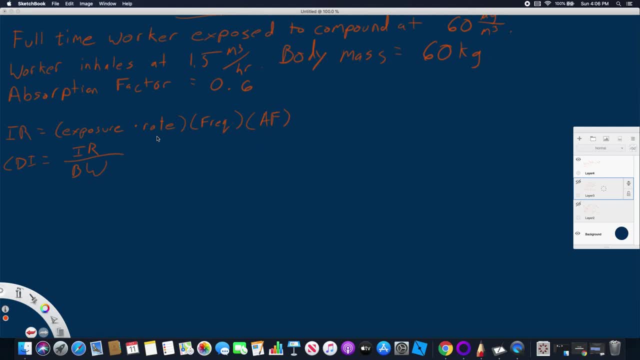 absorption factor, obviously, of only 0.6, and then our CDI is going to be our intake rate divided by our body weight, because body mass obviously is going to dilute. you know the risk here, so okay. so our IR intake rate, it's going to be 60 micrograms per cubic meter per hour. 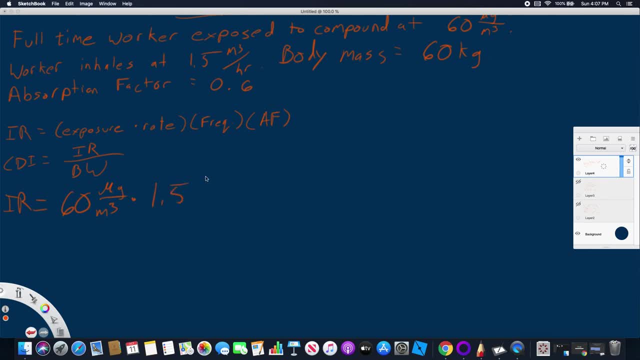 meter times our 1.5 cubic meters of inhalation per hour, and then we're just going to do conversion and then, since we're looking at our intake rate per hour, you know it's going to affect our exposure frequency because we're only breathing it, you know, during a work day or eight. 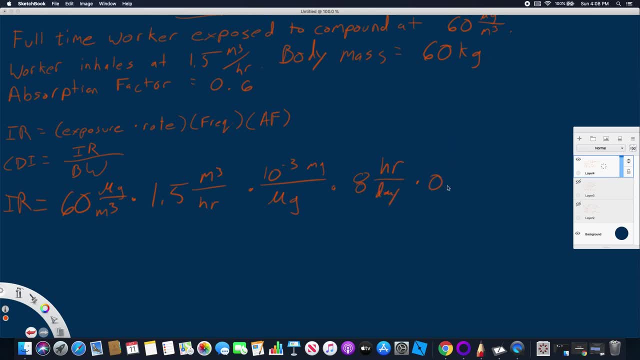 hour workday in this case- and that gives us 0.432 milligrams per day actually absorbed into our body. now now This again: this is just intake rate. it doesn't matter if you're a full grown adult or a baby, whatever, it doesn't matter in this case. 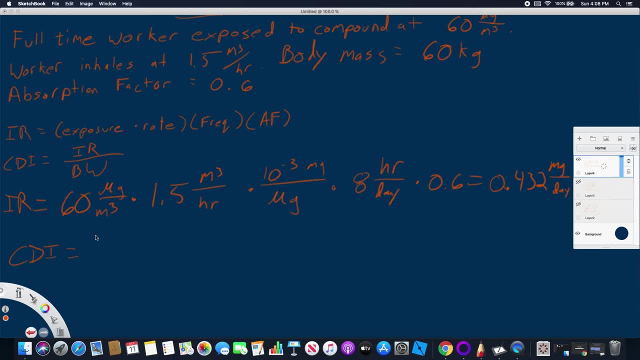 But when we look at chronic daily intake now, we're basically looking at the concentration in your body. So if we take our intake rate, divide it by our worker's body mass- sorry about that- then we have a CDI of 0.6.. 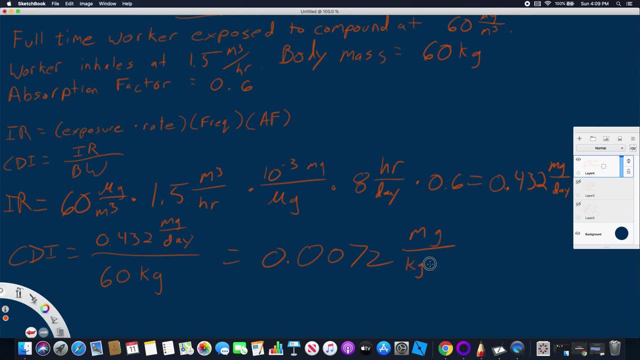 That's 0.0072 milligrams per kilogram day, And so you could use these numbers. obviously, you could be asked to calculate this. you could be asked to compare this to a NOEL. you could be asked to determine whether an